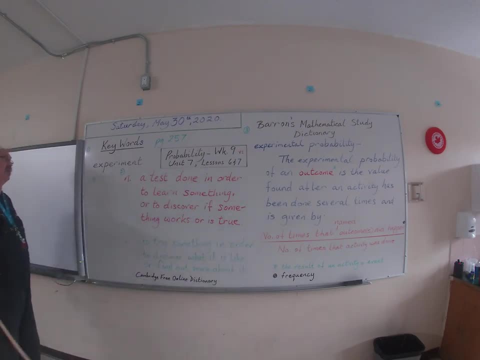 the Cambridge Free Online Dictionary And what it said was that as a noun- and in our textbook the word is being used as a noun- an experiment is a test done in order to learn something or to discover if something works or is true. So an experiment is a test done in order to learn something or to discover. 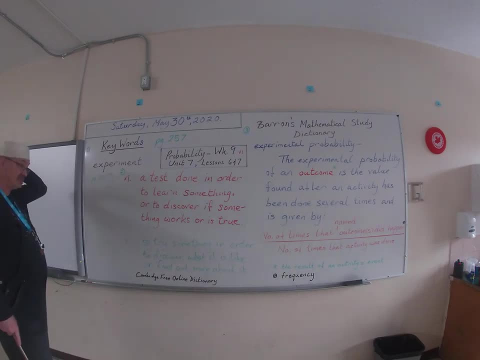 if something works or is true. That's the sense we're using in the textbook. As a verb, it means something fairly similar. As a verb, it means to try something in order to discover what it is like or find out more about it. 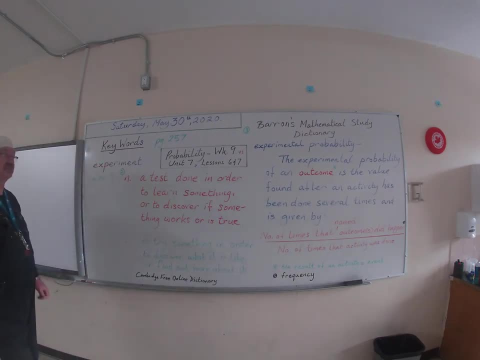 Okay, so that's a general definition of the word experiment. I then, of course, went to Barron's Mathematical Study Dictionary, and there was a definition for experimental probability, And what it said was: the experimental probability of an outcome is the value found after an activity. 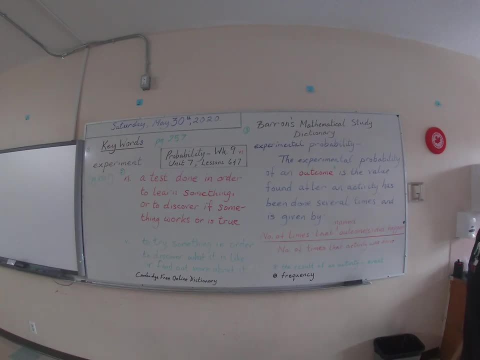 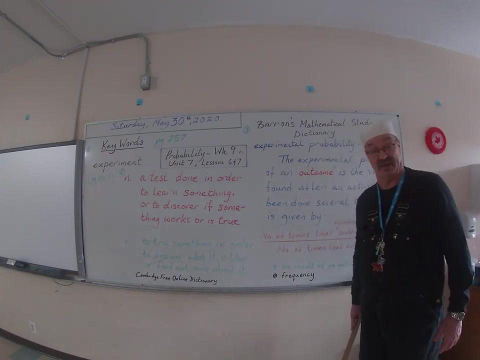 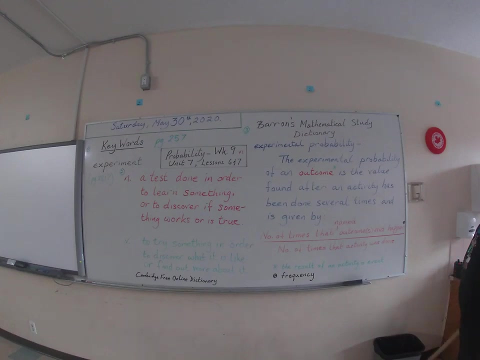 has been done several times and is given by. And when, in math they say it's given by, in that context, they mean usually that it's some sort of a formula. Before we move on, though, I'll just remind you that outcome is the result of an activity also known as an event. 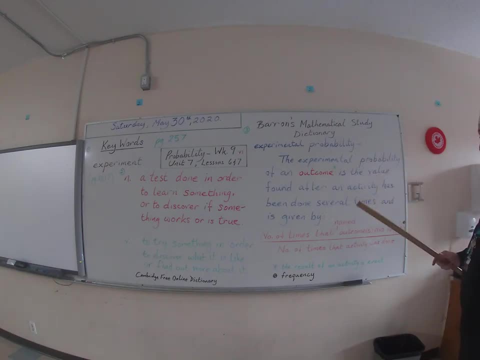 So the experimental probability. So the experimental probability of an event or the result of an activity is the value found after an activity has been done several times and is given by, And here we have the formula. So let's look at that formula. 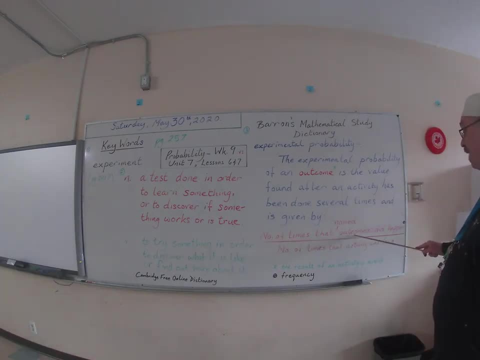